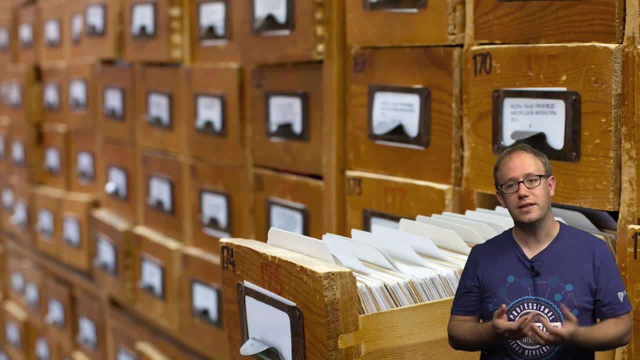 It's expensive to find data though, So we add indexes which make lookups faster. But if we do a bunch of joins then we have to perform query time index lookups for each and every join. That's fine if we've normalized into just a handful of tables. 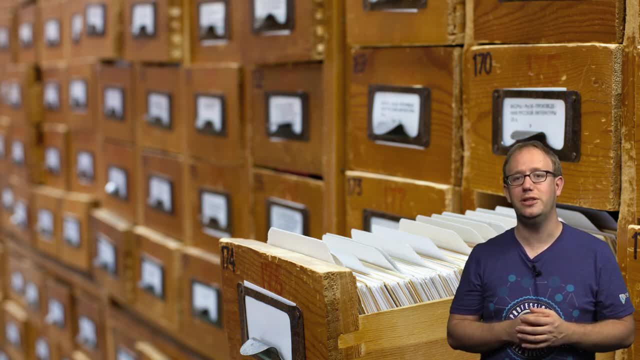 But what if it's 20 tables? Well, that's really expensive And it gets more and more expensive as your data size grows. Now, over the last 10 years, the cloud came along and things got a bit murkier, a bit less comfortable. 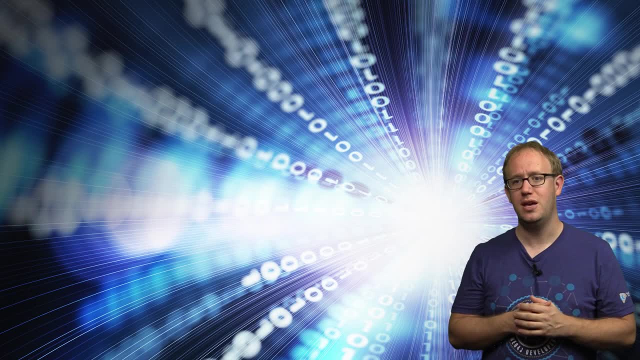 Why? Well, there's been a data explosion. Exabytes and exabytes. What do we do? We can store it on disk, for sure, But how do we make it easy to query? Can our database technologies keep up? Relational databases certainly couldn't handle this volume of data. 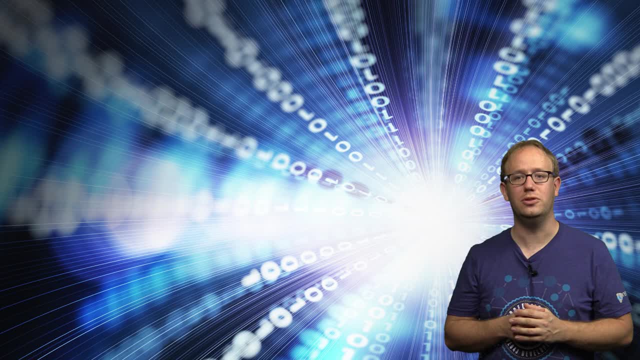 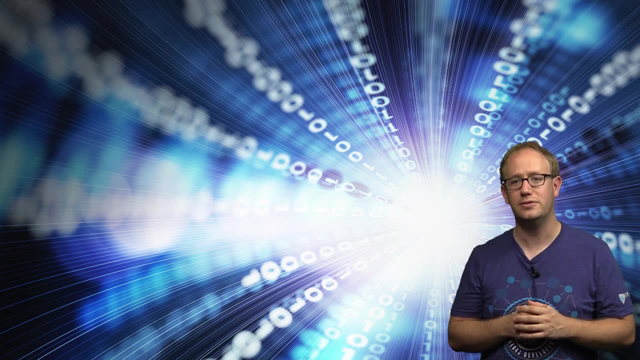 So innovation took off, and the NoSQL revolution was born. The NoSQL revolution was about making it possible to query more and more data. In order to do this, though, we had to discuss trade-offs. What trade-offs could we make that would make our databases faster? 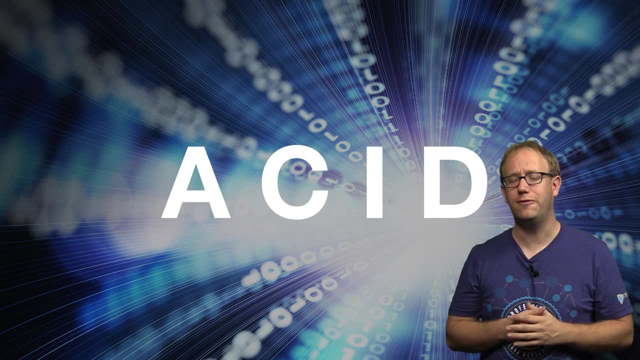 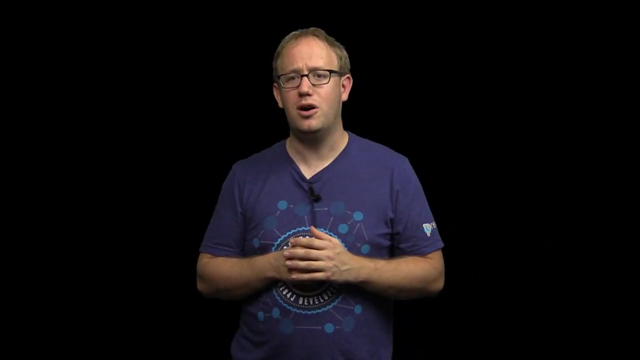 ACID was the first requirement to go. We threw it out the door. After all, with millions and millions of transactions, it's probably okay to lose a couple here and there. right Developer experience was also critical. How could we make it easier and easier to interact with large volumes of data? 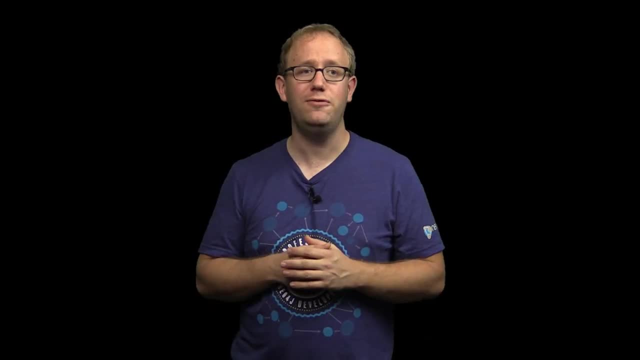 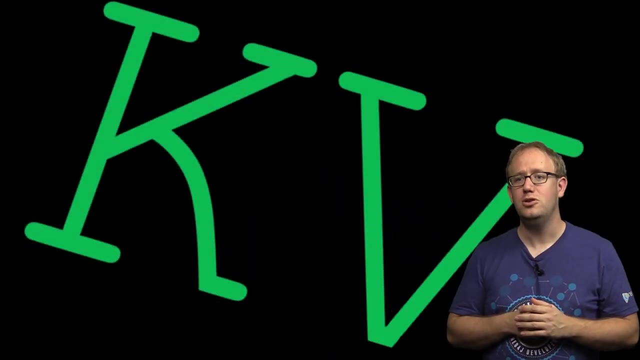 We needed to invent, or at least popularize, different interfaces for our developers. The most simplistic of these is a key-value interface. You store a value with a corresponding key. Later you can use that key to access the value, But the value is opaque. 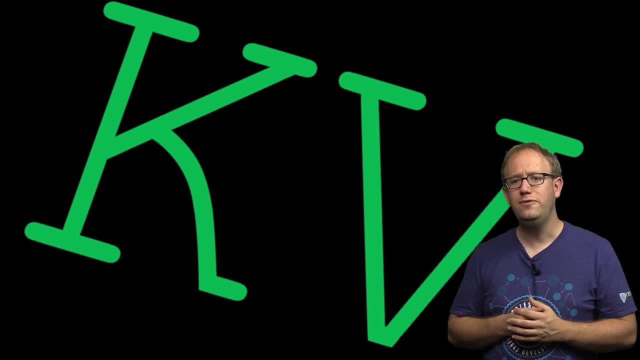 It's meaningless to the database. But what if you don't want opaque values? What if you want the database to index the values and make it easy to query based on the content? Well, that's what a document database is all about. It's a key that looks up a document. But you can also look up a document based on its contents, which are indexed for fast retrieval. Now what if we care less about the discrete bits of data and more about the relationship between our data? One document can reference another, but this isn't very performant or friendly from a developer perspective.